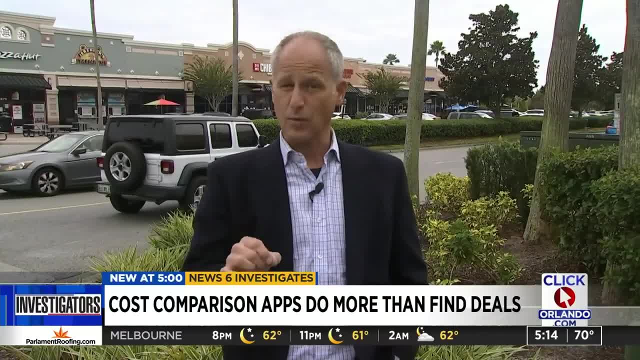 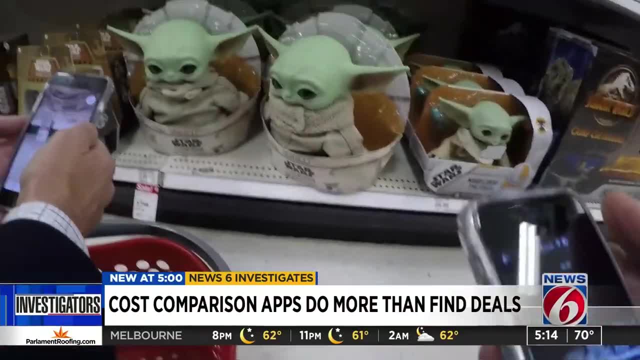 We wanted to see if they were getting results and if they were worth the price. Our shopping trip started with one of the most sought-after toys this holiday season: Baby Yoda. So this says it's $17.99 on sale, But was that $17.99 really a deal? 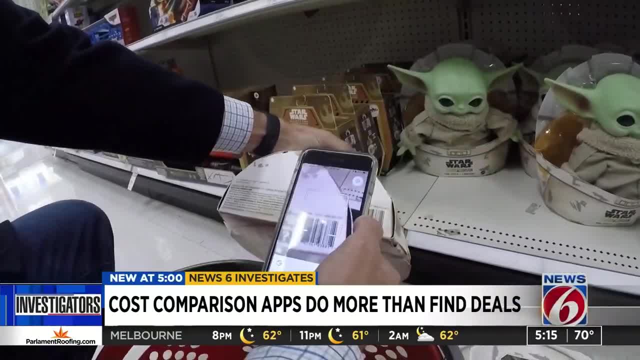 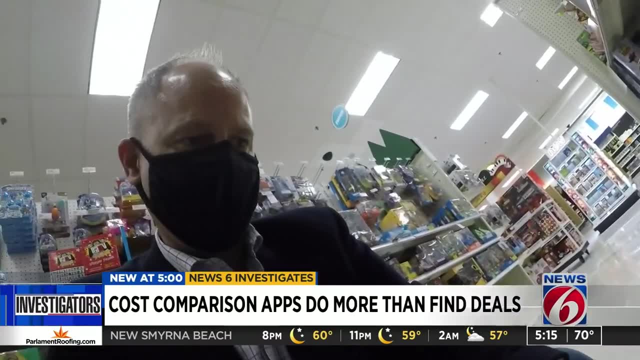 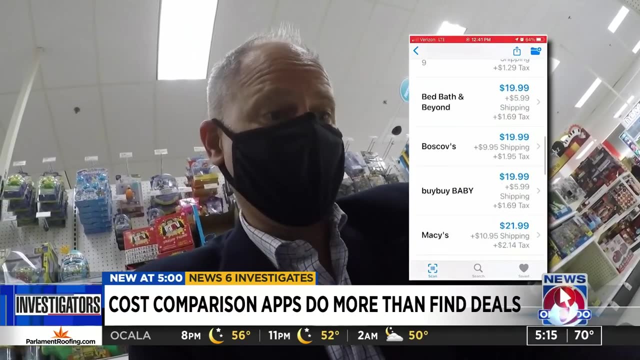 Well, using the ShopSavvy app, we scanned this little guy's barcode and the app showed it's scanning prices at other stores online. So it's as expensive as $24.99 at one store. You scan down $16 at ShopDisney, $18 at another store, $20,, $20,, $21,, $25. 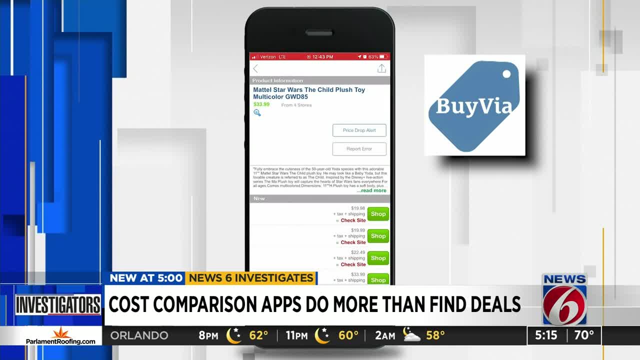 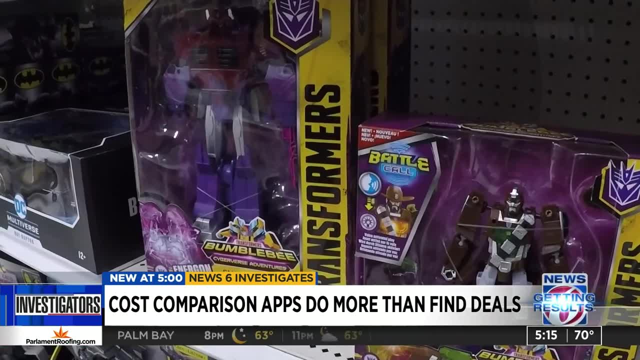 We also tried out Byvia, which offered coupons and showed us how much Baby Yoda was going for on eBay, which was about $33.99.. Next up this Transformer action figure retailing at this store for $29.99.. ShopSavvy's results. 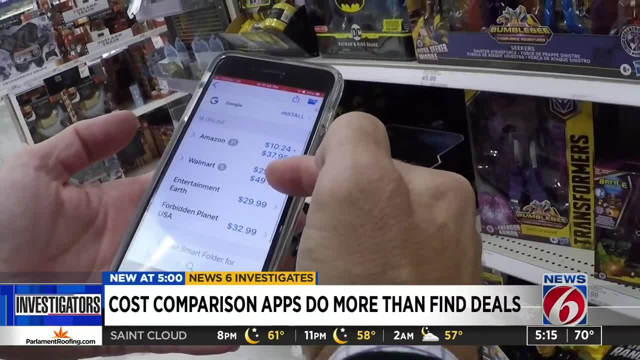 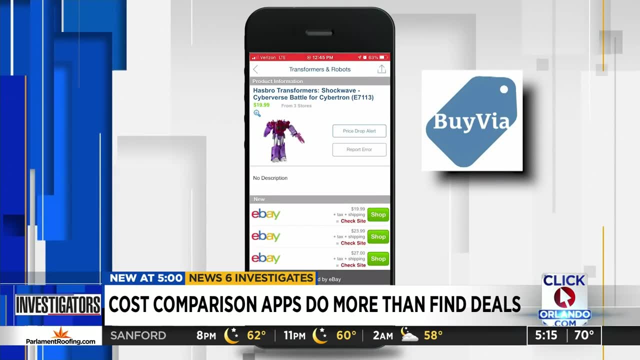 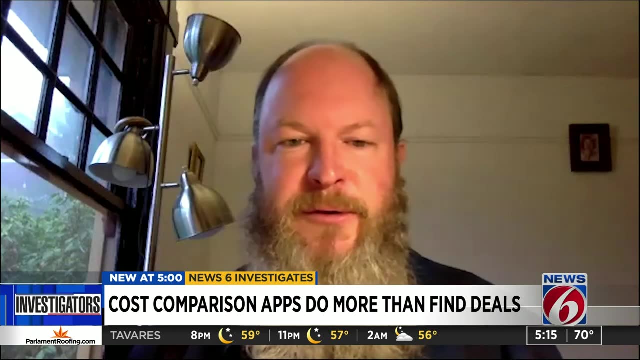 Amazon You can get it as low as $10.. Walmart about $30.. Forbidden Planet: $32.. Our scan using Byvia averaged about the same price on eBay. These apps, they can be really useful. Chris Minnick teaches app development at the University of Central Florida. 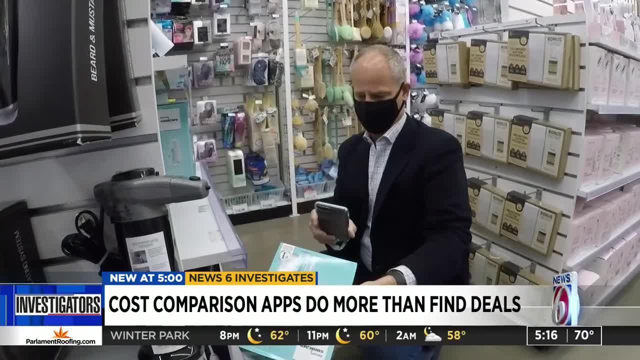 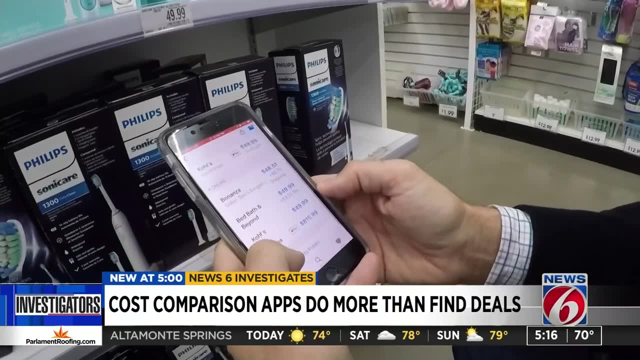 He says these apps and others like it collect these prices electronically from retailers all across the nation and online, And then they put them in the palm of your hand, usually for free. He says the retailers often pay these apps a referral fee. 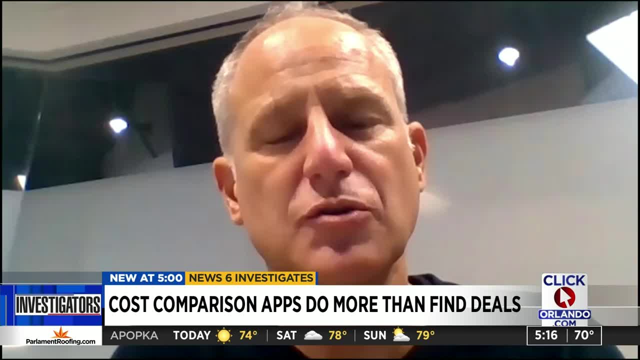 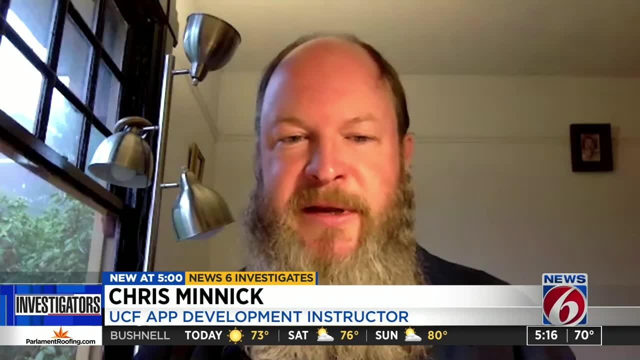 And that is how he says they make money. What are things that consumers need to look out for when they use these apps? It's collecting personal information. They're probably selling that personal information, And that would be another way that this app is making money. 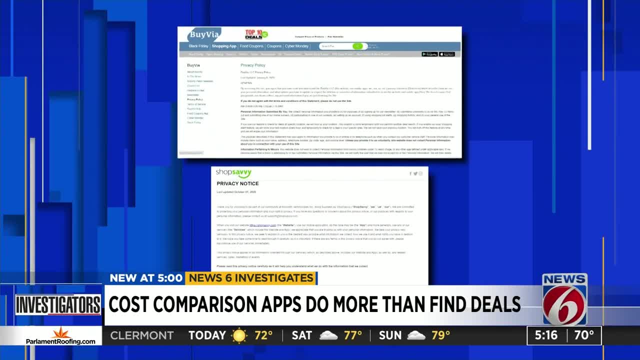 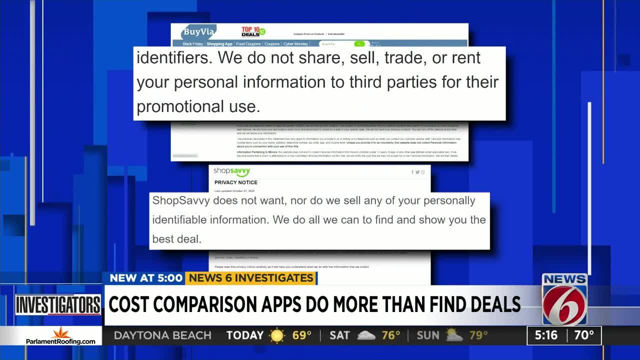 We checked the privacy policy for both of these apps. we tested and they say they do collect information. But both companies tell News 6 they do not sell that information. Minnick warns other companies May have different policies. So what happens when these apps just aren't right? 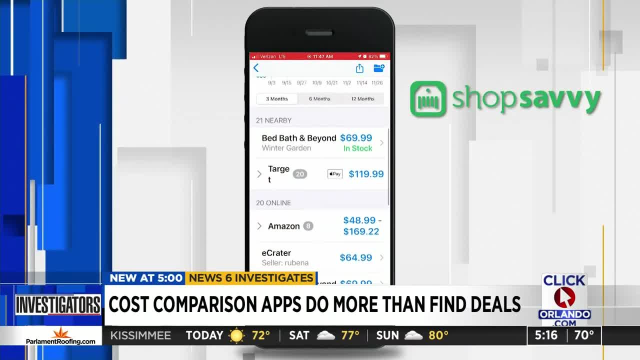 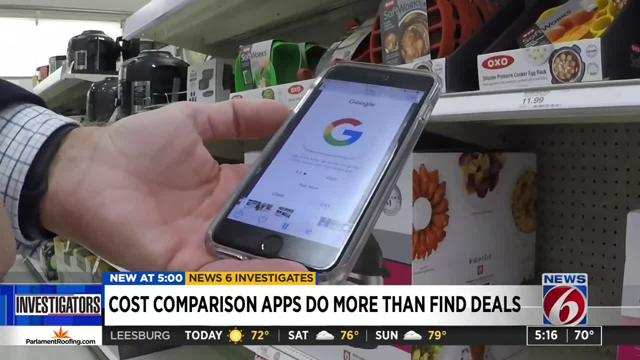 Take this Instapot, for example. The Shop Savvy app showed us it was $119 at Target. We went to Target and we found out it was actually on sale for $69.99.. We asked Shop Savvy about it and they claim it's rare.